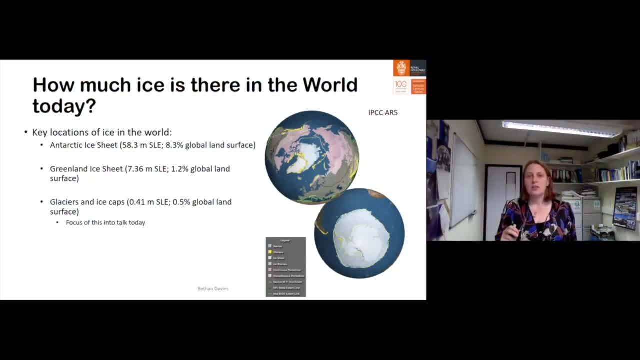 And if that melted, the world's sea levels would rise by about 7 metres. Glaciers and ice caps which are highlighted in yellow in this world map are actually a very small component of the world's ice, And if they all melted, the world's sea level would only rise by about 40 centimetres. 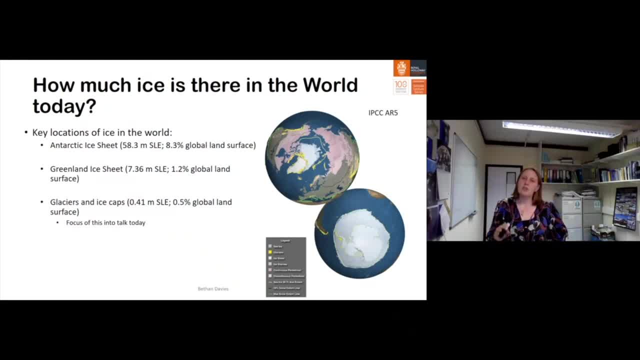 So although globally, glaciers Glaciers are only a very small store of ice, they're very important because they supply water for downstream areas, for irrigation, for hydropower, for domestic consumption and for industry. And as the glaciers recede, there are increased hazards in the mountain regions. 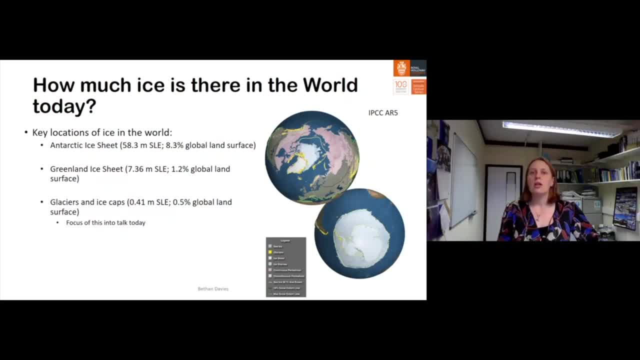 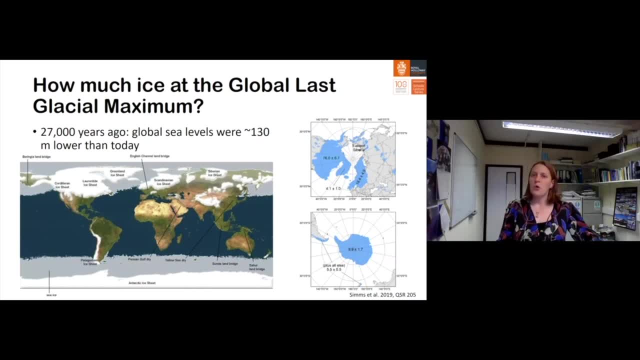 So today I'm going to focus on global glacier recession. How much ice was there in the world at the global last glacial maximum? Today we only have two ice sheets- the Greenland ice sheet and the Antarctic ice sheet, But 21,000 years ago there was a large ice sheet over North America called the Laurentide ice sheet. 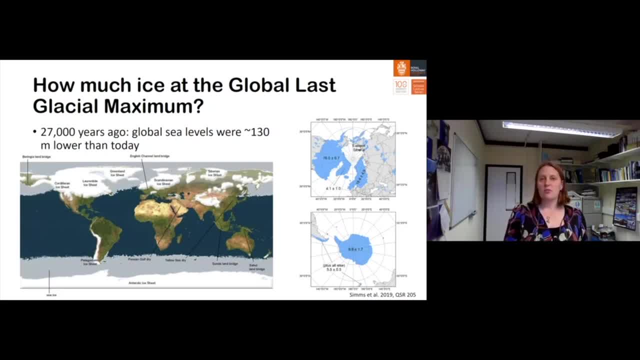 There was the Scandinavian and European ice sheet over Britain and Northern Europe And there was an enlarged. There was an enlarged Patagonian ice sheet, a Siberian ice sheet, And these large ice sheets lowered global sea levels by 130 metres. In blue here you can see the amount of sea level equivalent locked up in these ice sheets at the last glacial maximum. 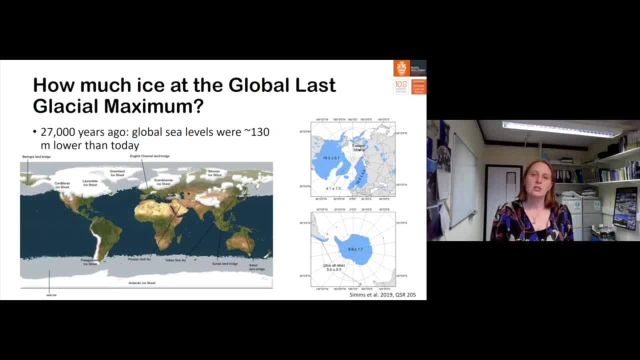 The Antarctic ice sheet only held an extra 10 metres of sea level equivalent, But the huge Laurentide ice sheet sucked up 76 metres worth of sea level. So glaciologists like myself, when we go to the beach and we dip our toes in the water, we don't see the sea. 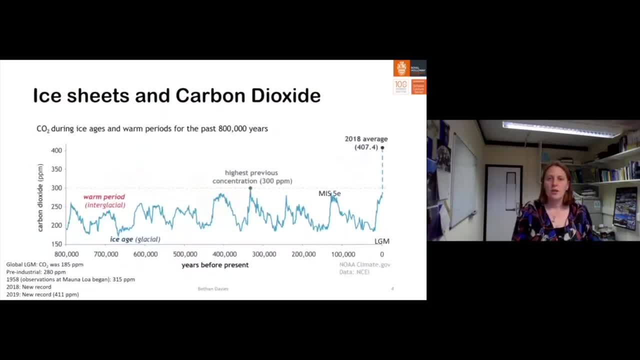 We see melted ice sheets. If we look at carbon dioxide, this is a measure of carbon dioxide for the last 800,000 years And you can see that over that time carbon dioxide has gone up And down, And when it goes down we have the growth of the global ice sheets. 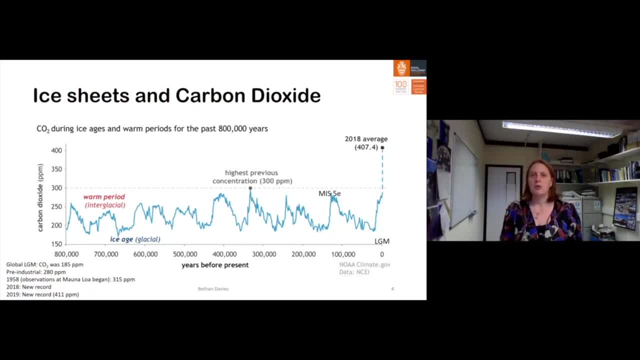 And when it goes up, sea levels rise and the ice sheets melt And over the last 800,000 years, global carbon dioxide has been between around 180 and 300 parts per million. Today, the global carbon dioxide is over 411 parts per million. 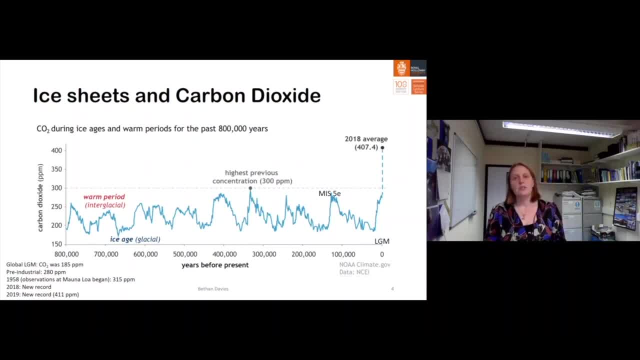 That is outstanding, That is outside the bounds of anything the world has seen over the last 800,000 years, If a rise in global carbon dioxide from 185 parts per million to 280 parts per million was enough to melt that huge Laurentide ice sheet. 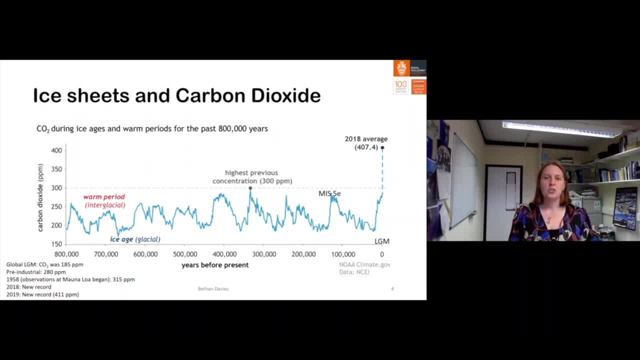 and destroy the Scandinavian ice sheet and remove the ice sheet over Britain. what will another 200 parts per million do? What will another 200 parts per million do to the world's climate? We are now in an unprecedented era of global carbon dioxide. 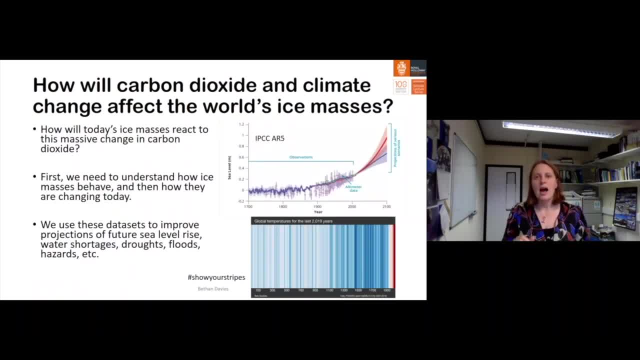 And the key question on everybody's mind is: how will this climate change affect the world's ice masses? Stripes here, the warming stripes. they show global temperatures since the year to the year zero, since the year zero AD, And you can see that the warming now is far greater than the global warming. 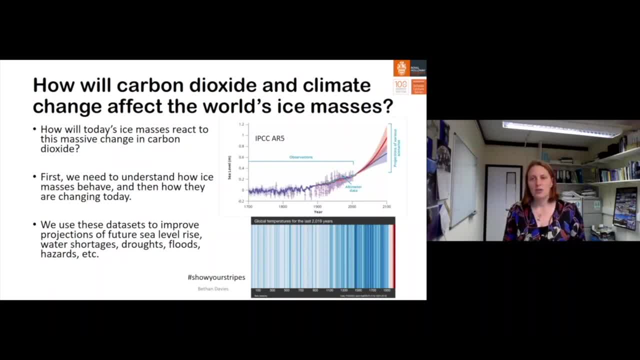 And you can see that the warming now is far greater than the global warming. And you can see that the warming now is far greater than the global warming. It's greater than anything we've seen in the past, And our projections of sea level rise to the year 2100 range between around 60 to over a metre sea level equivalent relative to the pre-industrial era. 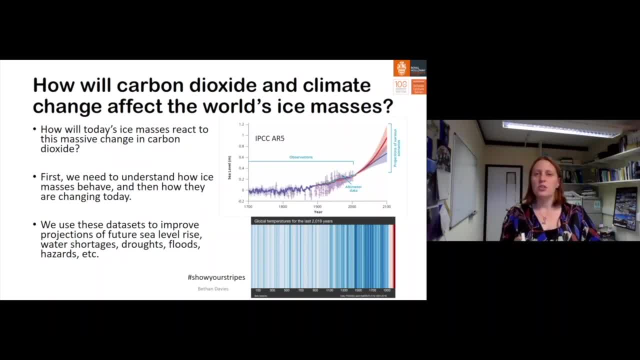 How are the world's glaciers going to respond to this? not only observed increase in carbon dioxide, but the future projected increases in temperature and carbon dioxide. We can use data sets like measurements of past climate change to make predictions of how glaciers will behave in the future. 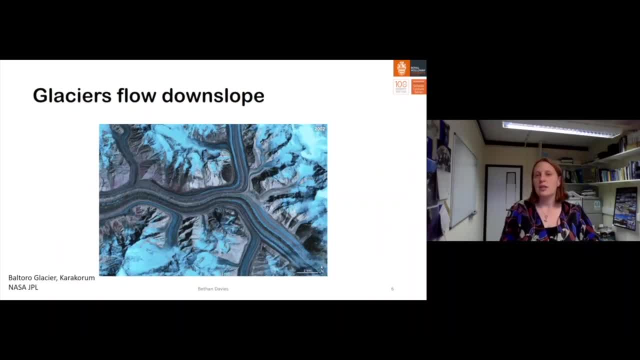 The key things that we need to take into consideration are how glaciers flow. Glaciers flow down slope. Ice flow is controlled by ice surface slope. Glaciers flow from highlands to the lowlands. They flow from the mountains down to the valleys. 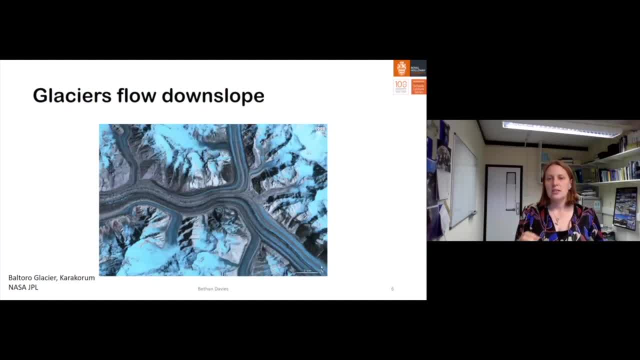 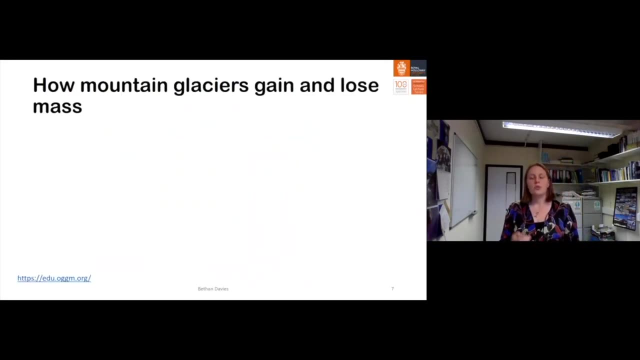 This is Baltoro Glacier in the Karakoram And you can see the glacier moving as it's oozing downslope. It's like a very thick, sticky liquid and it can flow under its own weight. Mountain glaciers also gain and lose mass. 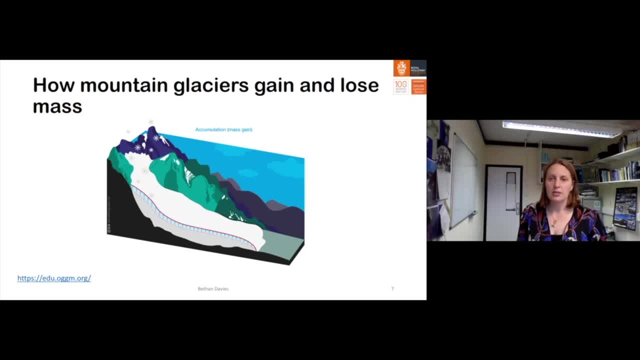 Firstly, mountain glaciers gain mass through the process, the process of accumulation. Accumulation is all the snow and precipitation and rain and frozen frost that add mass to the glacier. Even rockfall onto the ice surface could be considered accumulation. So each year glaciers accumulate mass. 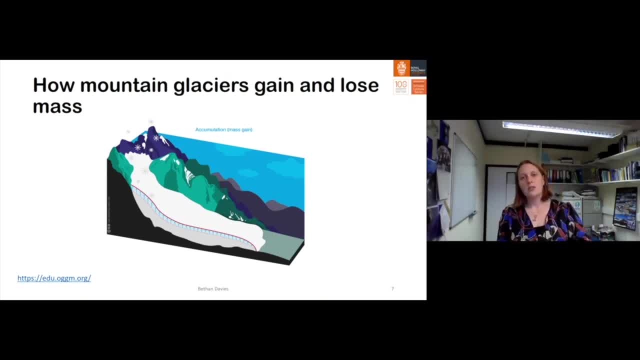 They tend to accumulate more mass in their upper parts because it's colder there And so more of the precipitation is falling as rain Each year. glaciers also lose mass, And the process by which glaciers lose mass is called ablation. In Europe, in the Alps, glaciers tend to gain mass in the winter and lose mass by melting in the summer. 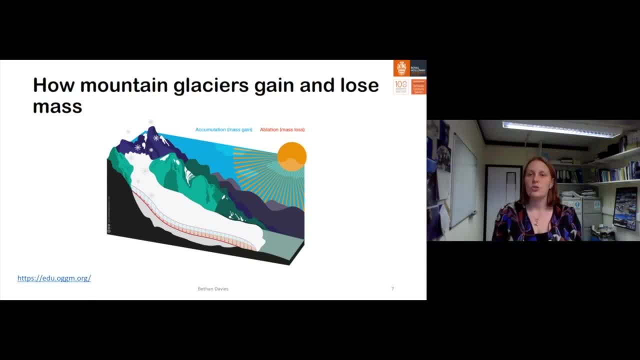 In parts of the world where glaciers terminate in lakes or in the sea, they can also lose mass by carving icebergs that float away into the ocean. So each year glaciers gain mass or accumulate mass, And they also lose mass, or they undergo ablation as they melt. 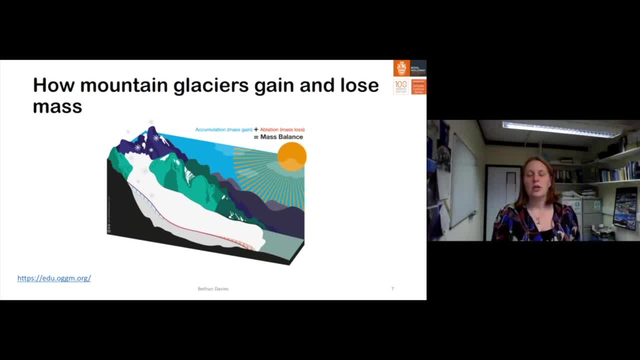 The balance between accumulation and ablation is the mass balance of the glacier. You can think of it a little bit like a bank account. Each year you have a certain amount of money coming into your bank account and a certain amount of money going out of your bank account. 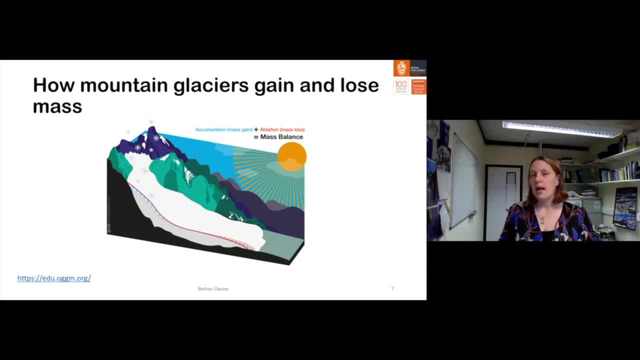 If you have more money coming in than you have going out, your bank account will grow and you'll be richer. If you spend more money than you gain, then your bank account will steadily get smaller And every year your bank account will shrink and you'll be poorer. 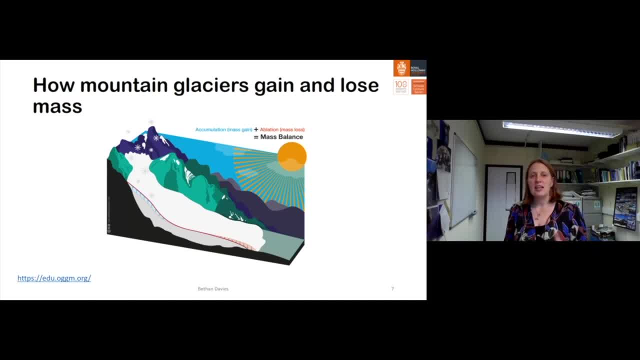 So glaciers are the same. Each year. they gain and lose mass. If they gain more than they lose, then the glaciers have a positive mass balance and they will grow. If the glaciers lose more than they gain, then they will have a negative mass balance and they will shrink. 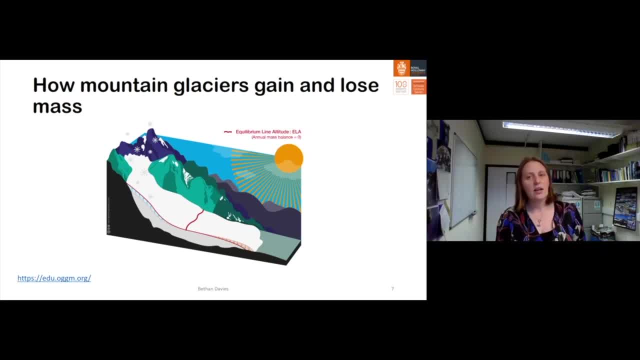 The line in between net gain and net loss is the equilibrium line. So the equilibrium line, the gain is equal, is equal to the loss. So here you can see, above the equilibrium line, we have net gain to the glacier. This is the accumulation zone. 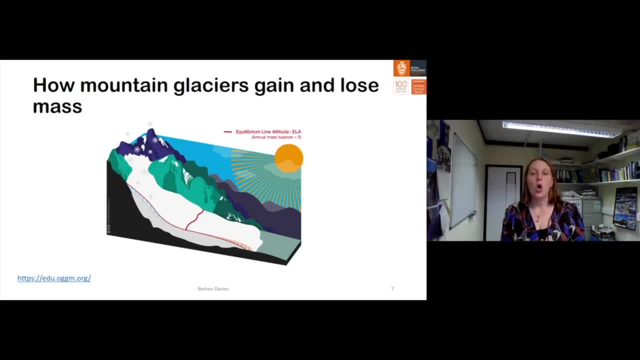 Below the equilibrium line we have net or loss. This is the ablation zone of the glacier. If temperatures rise due to climate change, the equilibrium line altitude will grow, The area of the glacier with net mass gain will shrink and the area of the glacier with net mass loss will grow. 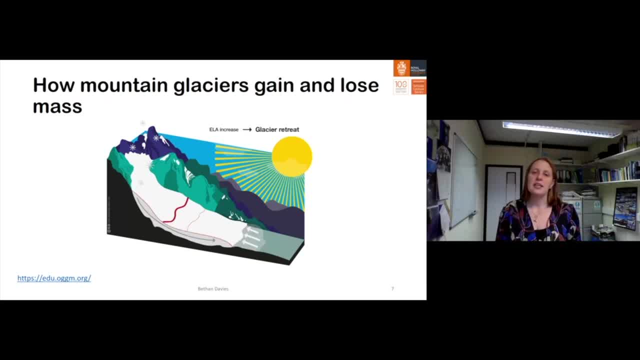 If this happens, the glacier will lose more mass than it gains and, as a result, the glacier will shrink. So here, although the glacier is continuing to flow downslope under the force of gravity, the accumulation area has shrunk And the glacier is retreating. 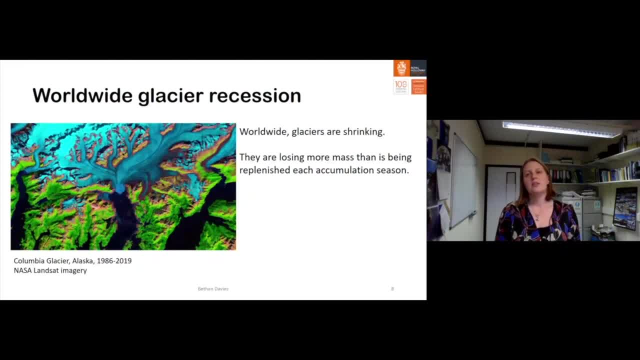 Worldwide, glaciers are losing more mass than they are gaining. This is Columbia Glacier in Alaska, a very, very large glacier in Alaska, And it has been steadily retreating These satellite images, and there's one for every year between 1986 and 2019,. 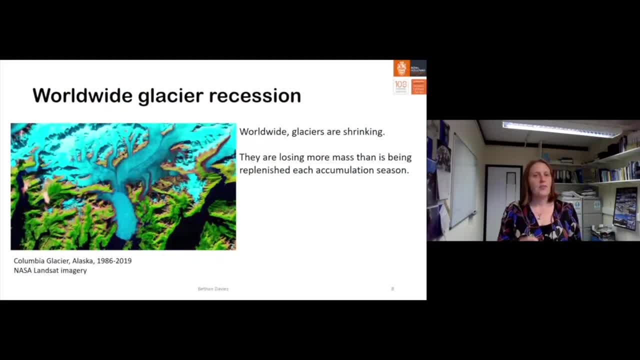 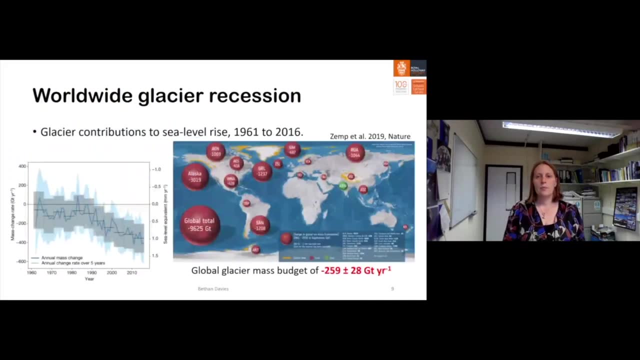 show the recession of the glacier through time. This pattern of worldwide glaciation is repeated all over the world, as glaciers are losing more mass than is being replenished in each accumulation season. Since 1961, worldwide glaciers have lost 9,625 billion tons of ice. 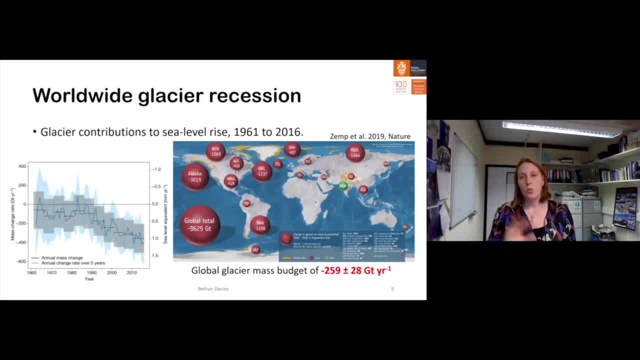 These circles show how much ice has been lost. So the global total is 9,625 gigatons And a gigaton is a billion tons, And you can see that we're also losing substantial amounts of ice from places like Alaska, the Southern Andes, from the glaciers around the Greenland ice sheet. 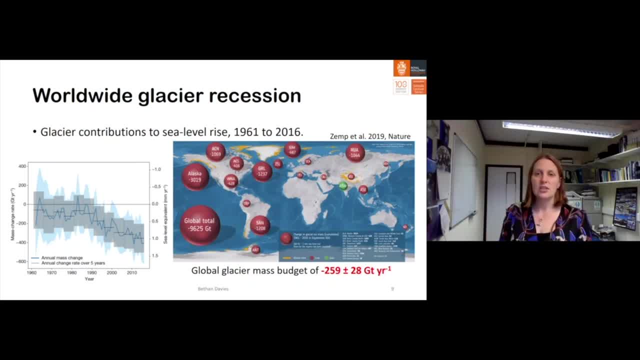 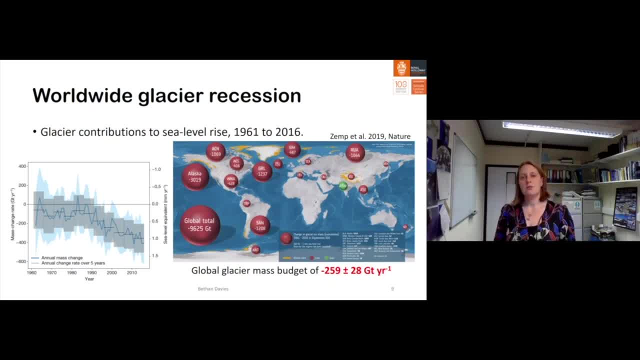 And that equates to around two-thirds of a millimeter of sea level rise every year, just from global glacier recession. And you can see in this graph that that contribution to global sea level rise has been accelerating over time And it's now nearing a whole millimeter per year. 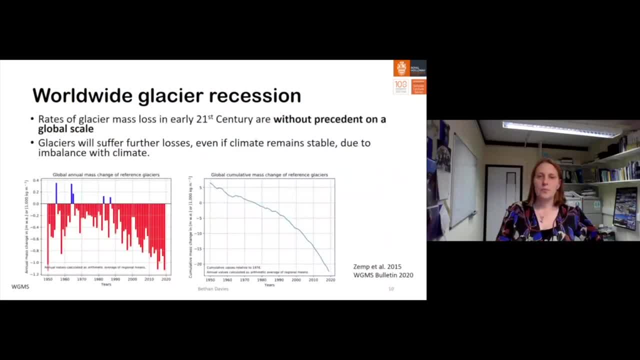 just from global glacier melt, And it's now nearing a whole millimeter per year just from global glacier melt. These rates of glacier mass loss from the year 2000 onwards are without precedent on a global scale. We have not seen this behavior before. 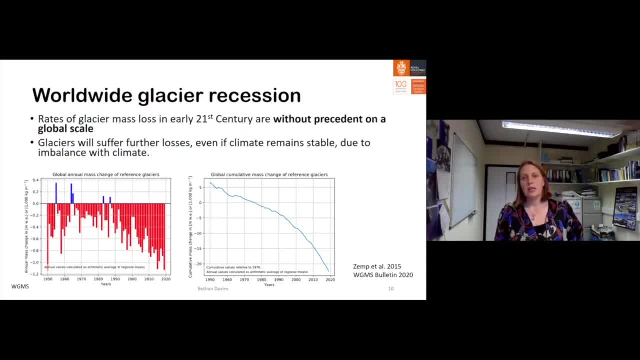 And glaciers will suffer from further losses even if the climate remains stable, because they are not yet in balance with the climate. So the glaciers will continue to recede even if the climate remains stable And the climate stops warming. Here on the graph on the right you have cumulative mass change of certain reference glaciers. 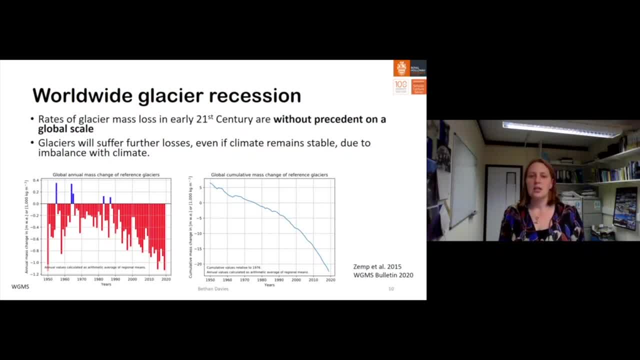 that have been studied every year for the last 60 to 70 years And you can see that the cumulative mass change is growing ever more. These glaciers are shrinking every year And for these reference glaciers, the histogram with the blue bars and the red bars 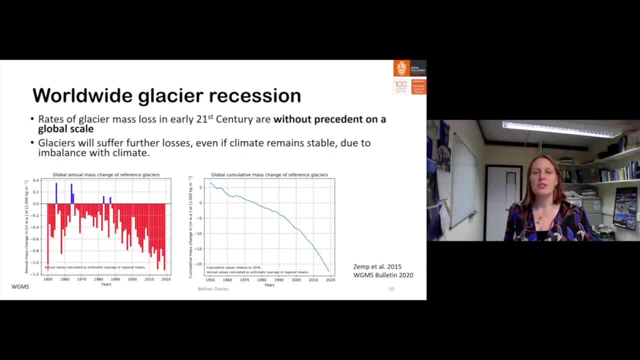 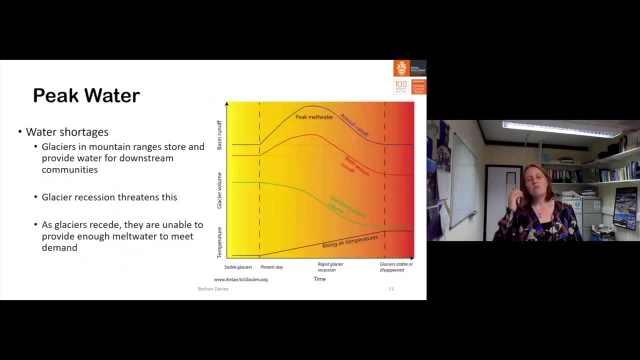 shows that the annual mass change is becoming increasingly significant. Each year, these glaciers are losing even more mass than the year before. So the glaciers are continuing to shrink And this has really important connotations for people who rely on glaciers for meltwater. We can think of the concept of peak water. 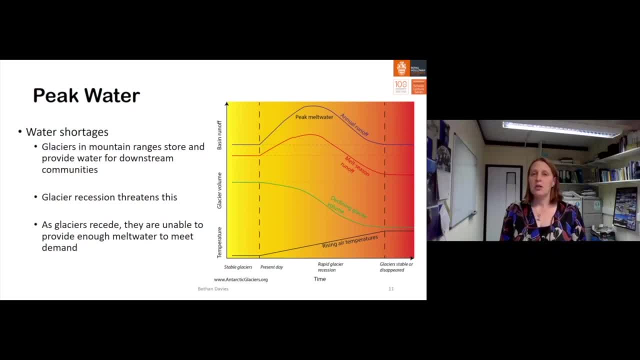 In the first half of this year, glaciers melt And as they melt, people downstream use that meltwater in their daily lives In Europe. in Switzerland, for example, some of that meltwater is used for hydropower. In the Himalaya, a lot of that meltwater is used for crop irrigation. 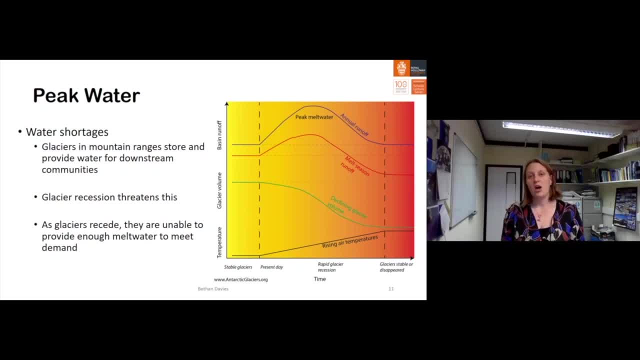 And in the Andes the water is used for irrigation, industry and hydropower, So it's really useful And around a third of the world's population is using it. And around a third of the world's population is using it. 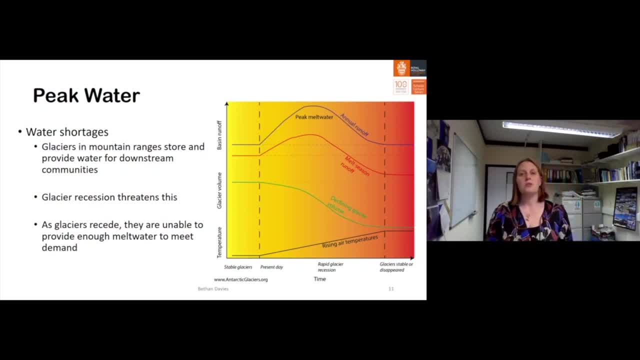 And around a third of the world's population is using it. It's living in regions that receive meltwater from glaciers, And as the glaciers shrink, the amount of meltwater they produce eventually starts to shrink too, And we can think of this as the concept of Peak Water. 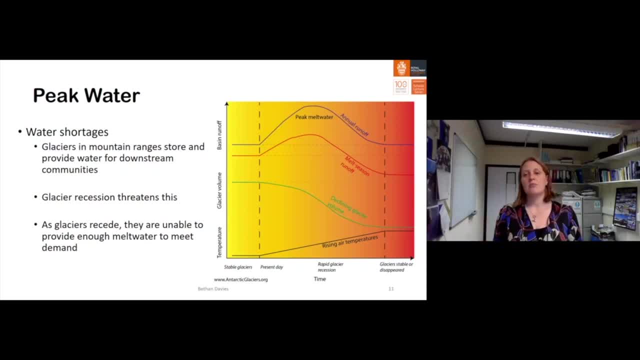 In this graph, along the bottom we have rising air temperatures through time. In the green line we have glacier volume. In the green line we have glacier volume. glacier volume is declining. The melt water from the glaciers rises annually as the glaciers start to shrink, but then starts to decrease and the annual runoff. 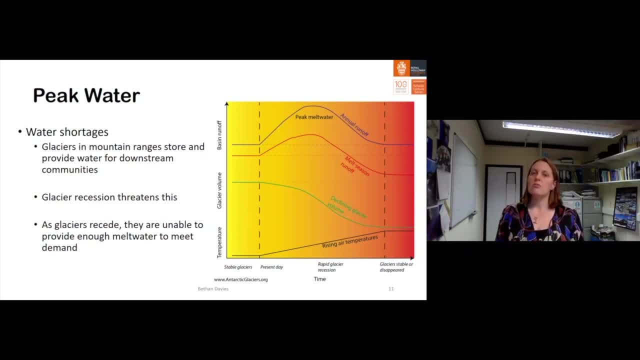 which is all the runoff from all the precipitation, as well as the runoff from the glacier. you can see that you have a peak in that and then it decreases, and so we have peak water, when we have the maximum amount of water available, and that's a great time. you can plant more avocados, you can grow more crops. life is. 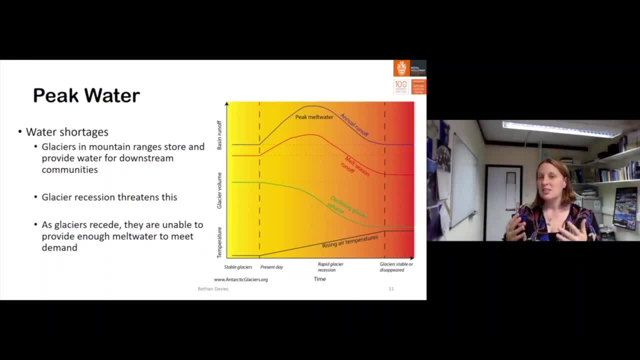 good. but as the melt water starts to disappear, you suddenly find yourself living in an area with severe water shortages, especially if there is a drought and there is less rainfall. The glaciers are no longer able to provide their buffer to the glaciers. This is a suffering role which protects people from droughts and changes in. 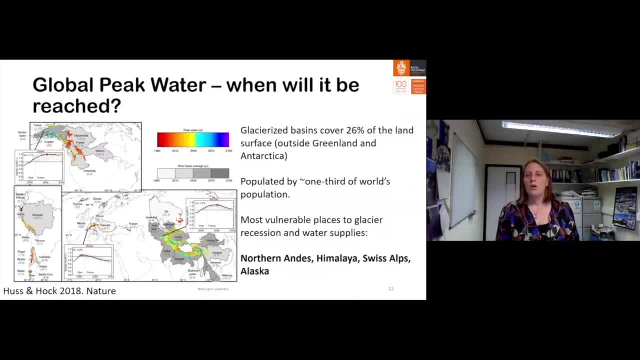 precipitation. Global peak water will be in a different year depending on where in the world you are. It's dependent on the volume of the glaciers. Areas with smaller glaciers like Peru and Bolivia, and the tropical Andes have already experienced peak melt water and parts of 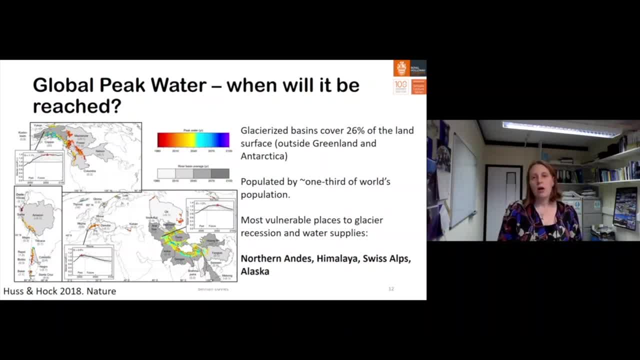 Alaska, peak melt water will come in some decades because the glaciers are very large here, but then we have the Fraser and the McKenzie and the Columbia River, and these rivers, these glaciers, have already reached peak melt water. In the Himalaya, peak water will be reached around the year 2030 to 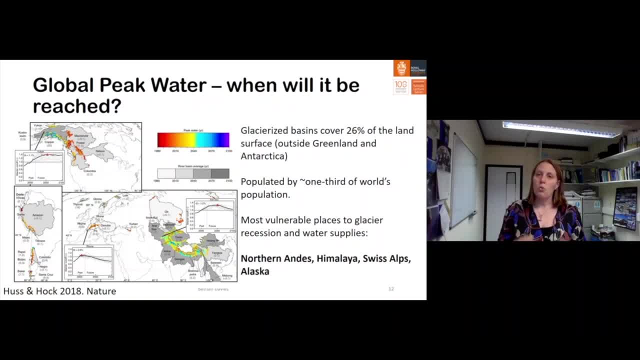 2040, so in the next two or three decades, water in the Himalaya will decrease. In this sort of weather, it will not only be notifications, but also at the, the city and the water level as a whole In the northern majesty, in the Libertarian 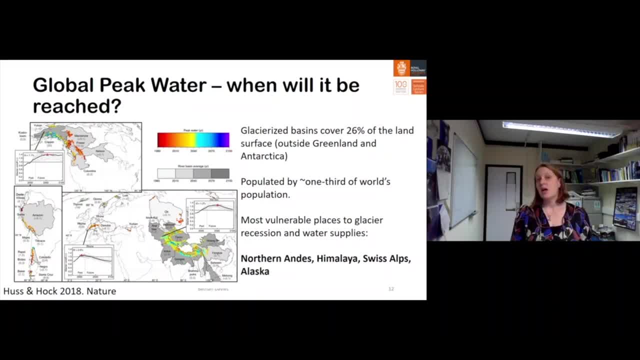 Cr Mi lies the fifth most exposed glacier in water history And theokola In the northern majesty, in the Libertarian Cr Mi lies the fifth most exposed glacier in water history And the Dromansfel is the 3rd most aلى heavenly to find here. 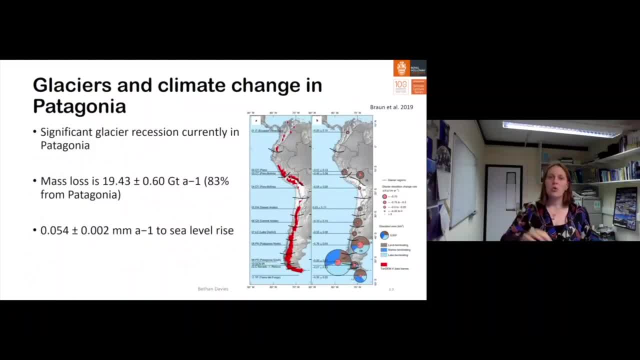 In the northernき usage f the people of North Africa have alwaih. mystery chambers are first designed by the Estereí Group of Historic States, the Global Geographic and Geographic Special Research Team, ERI, Mac Collicle, and this meant that the 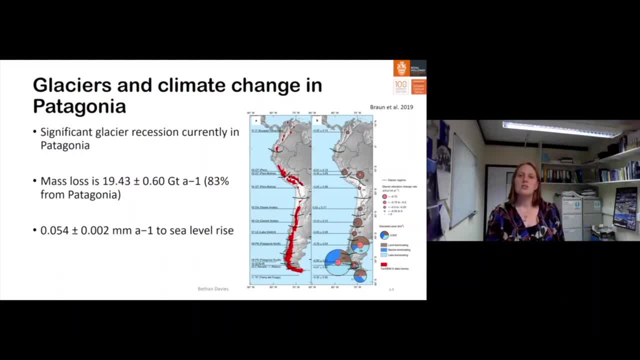 Southern Andes, contributing around 19 billion tonnes of ice to sea level rise every year, which is around half a millimetre of sea level rise. If you look at panel B in this map, the size of the pink circles is the rate of mass loss from the glaciers. 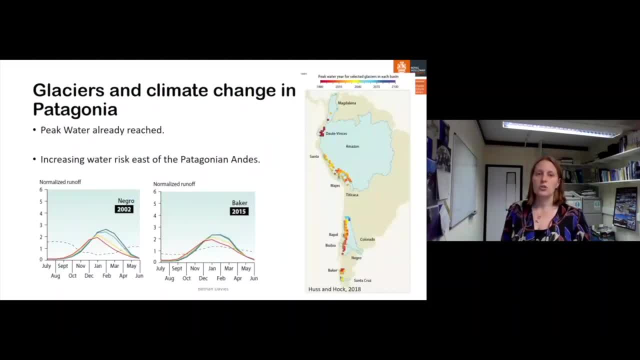 The bigger the circle, the more mass is lost. In these regions, peak water has already been reached. For example, the Negro River and the Baker River have already reached peak mill water and the water is now declining. In Peru, the peak water was reached in the 80s and water shortages are now a common occurrence. 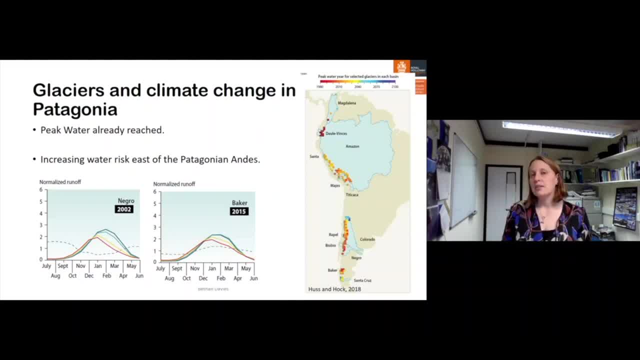 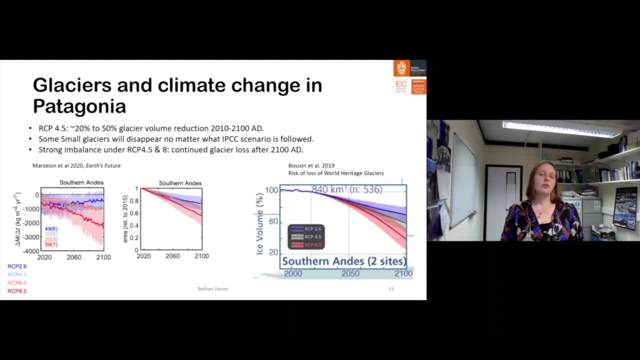 This is increasing water risk east of the Patagonian Andes. If we continue on our current trajectory of evolution, we can expect to lose more than 20% of global emissions. This is approximately equivalent to the IPCC scenario: RCP 4.5.. 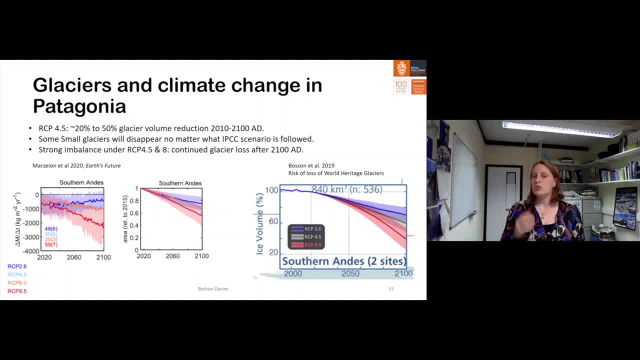 If we continue on this, we can expect to lose globally between 20 and 50% of glacier volume by the year 2100.. RCP 2.6,, which is represented in these graphs by blue lines, is approximately equivalent to the Paris Agreement. 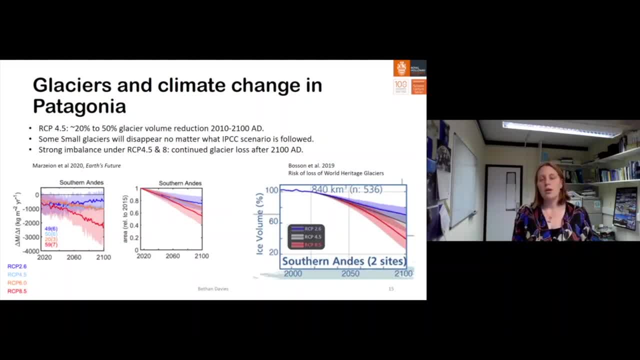 and will see us limiting our emissions. If we follow RCP 2.6 and follow a high mitigation scenario with reduced carbon emissions, then we will retain the majority of the glacier ice. These graphs show the projected glacier volume in the southern Andes. 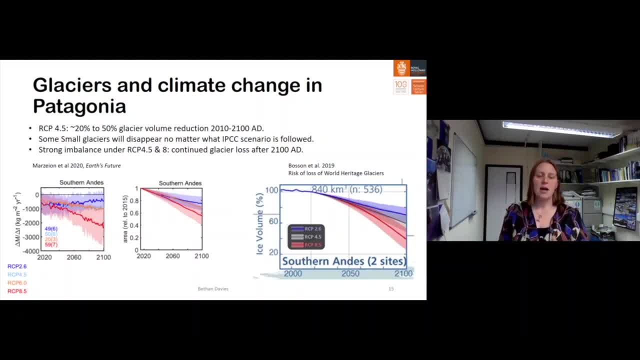 We have area in one and mass balance in the other. You can see that the projected area is the volume of the glacier. The projected area is around 80% remaining under RCP 2.6 and around 50% remaining under the highest end scenarios. 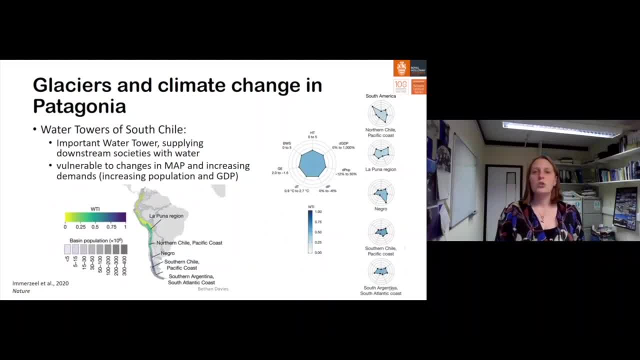 The glaciers in Patagonia are an important water tower. A water tower is a mountain region and it's a mountain region with glaciers on it. That's how we define a water tower. In this project that I was involved with, we have a large number of water towers in the southern Andes. 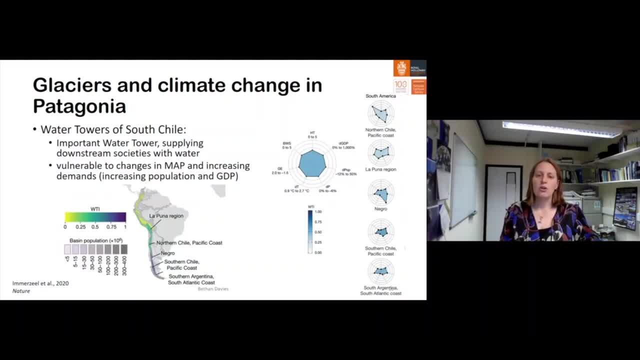 We have La Puna, Northern Chile, Negro, Southern Chile, the Pacific Coast and Southern Argentina. They're coloured according to the Water Tower Index. The Water Tower Index is the amount of water produced and supplied by this water tower versus the amount of water demanded. 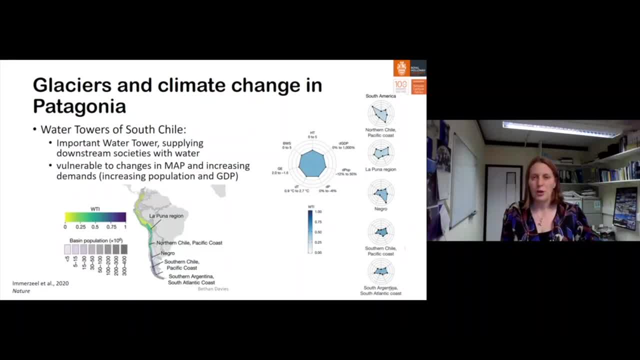 The amount of water demanded from the water tower. We demand water in terms of for irrigation, for industry, for natural resources, for the forests that grow in these regions. These water towers in the southern Andes are vulnerable. These spider diagrams illustrate the vulnerabilities of these water towers. 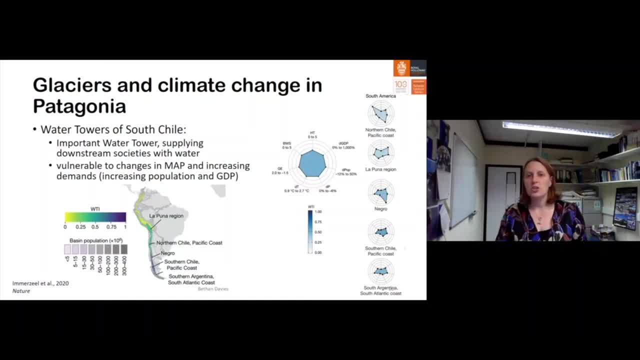 We go from the top from 12 o'clock. We have hydro-political tension, changes in GDP, changes in population, changes in precipitation, DET is changes in temperature, GE is government effectiveness and BWS is baseline water stress. You can see that in South America. 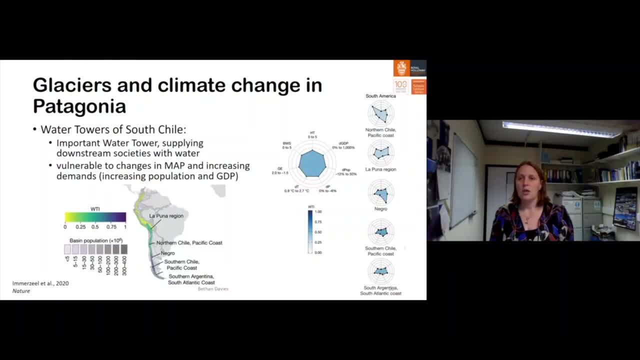 the water towers are vulnerable to baseline water stress, but also significantly to changes in precipitation. Changes in precipitation, which are projected to occur under climate change scenarios and which are exacerbated by changes in the winds in Patagonia, drive rapid glacier recession. 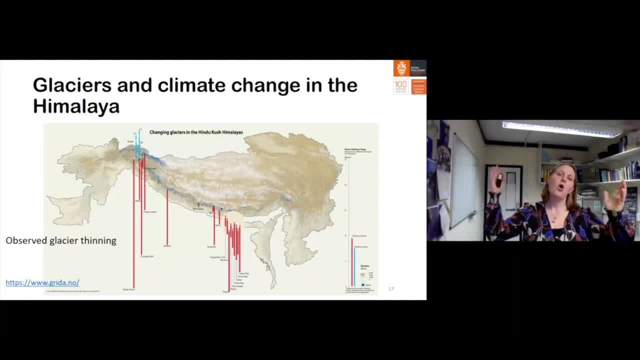 Let's move to the Himalaya, the third pole, the highest mountains in the world. These glaciers, uniformly, are thinning. Here we have the red bar charts. These reds show the thickness reduction of glaciers across the Himalaya Where the bars are longest. 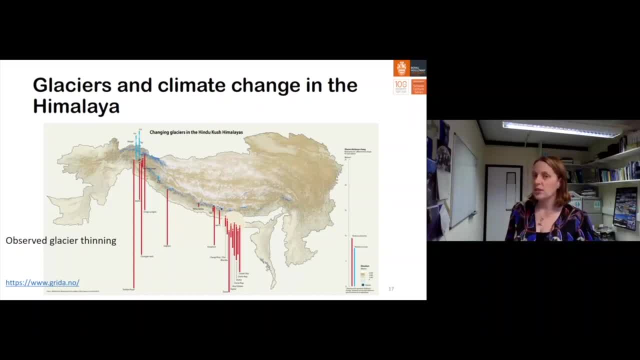 that's where we're seeing the most significant changes in glacier thickness. If the bars are blue, then the glacier is thickening, so it's gaining more mass than it's melting, But this is only restricted to a very small number of glaciers. 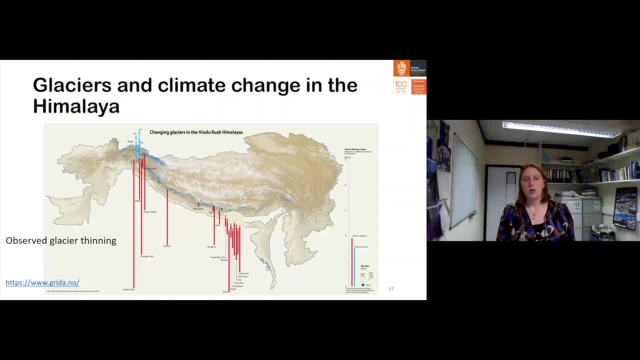 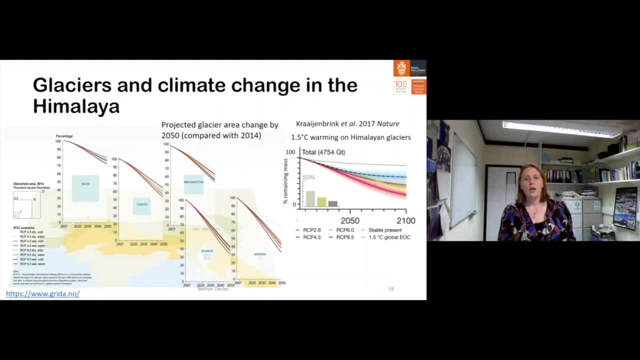 which are affected by changes in the monsoon. Across the rest of the Himalaya, the glaciers are shrinking and thinning. If we project how much glacier area we'll have by 2050, and we're again looking at RCP 4.5 to RCP 8.5,. 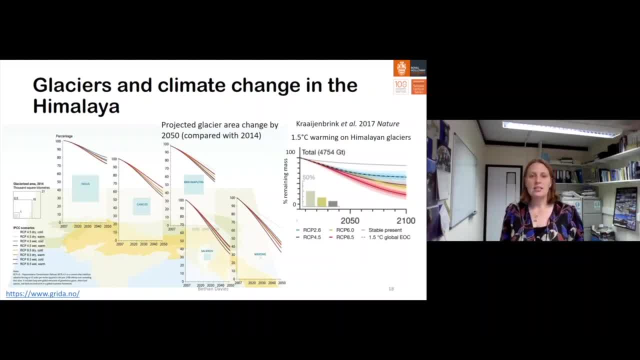 then we can expect to lose between 20 and 40% of our glacier area in the Himalayas. And yet if we limit climate change to 1.5 degrees C, this study shows in this graph on the right here- this study shows that under RCP 2.6,. 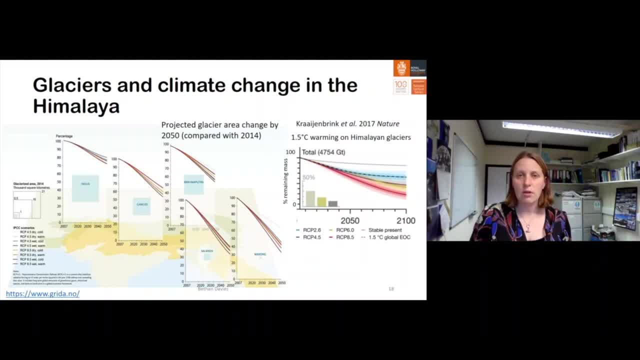 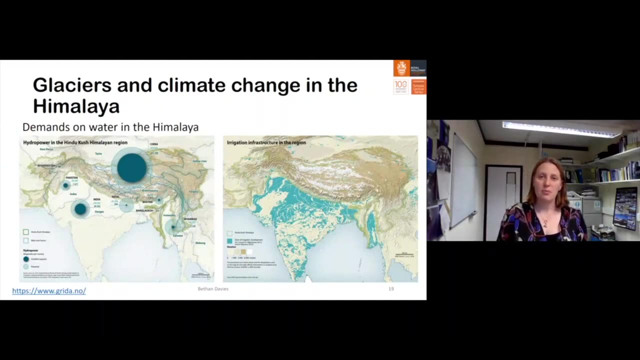 which limits warming to 1.5 degrees centigrade, we can expect to retain most of the ice volume in the Himalaya. This is really important because 235 million people live in areas downstream of the Himalaya. This is hydropower. 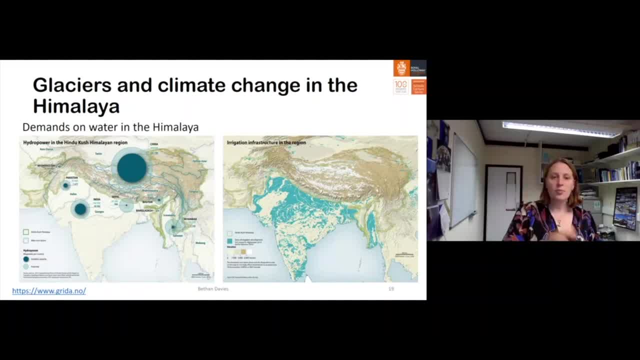 Hydropower in the Hindu Kush And you can see the dark blue circles is the installed capacity of hydropower and the light blue circles is the potential capacity for hydropower. These glaciers in these regions are really driving hydropower in the Himalaya. 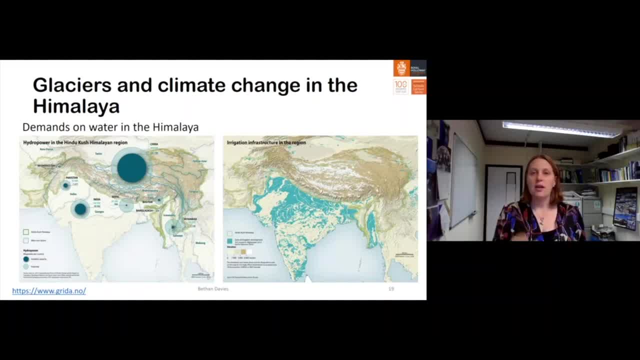 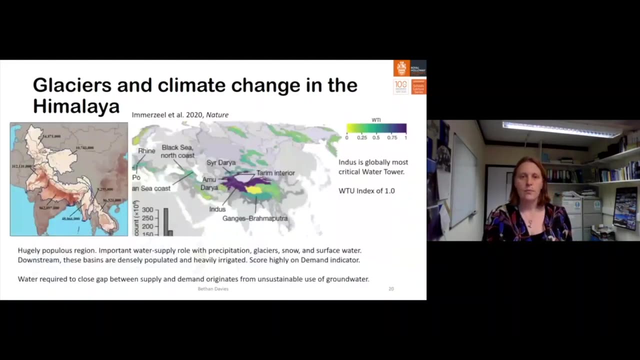 And in the other map we have infrastructure for irrigation And the blue areas here are zones of irrigation development. And again downstream of the Himalaya we have substantial irrigation development. That means that the glaciers in the Himalaya are a critical water tower. 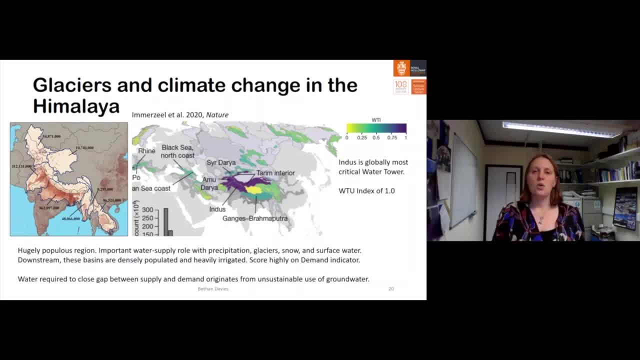 The Indus and the Tarim interior are considered the world's most important water towers. That is because there is a huge population of people, hundreds of millions of people, living downstream of these water towers. These water towers are used for irrigation, for hydropower, for industry and consumption. 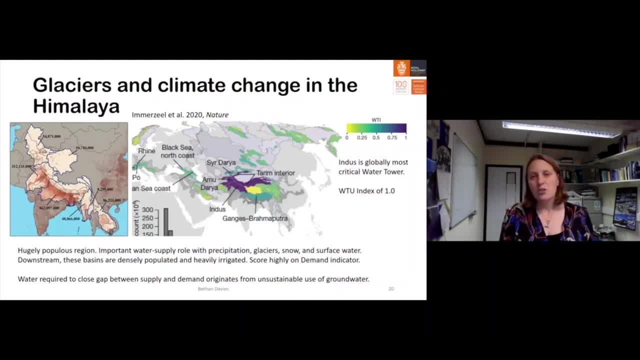 So there is a high demand for the water Already. there is more demand for water than there is supply In these parts of the world. we already see that the water gap between the supply of the water and the demand for the water is filled with unsustainable water. 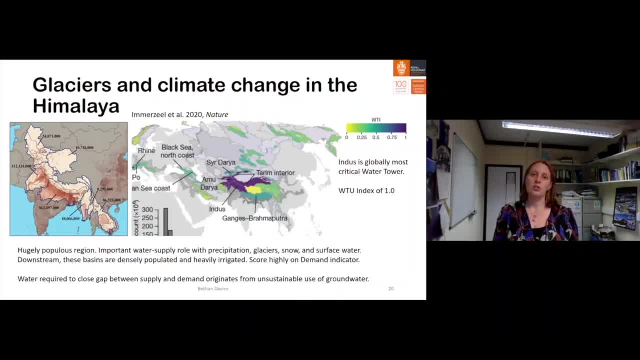 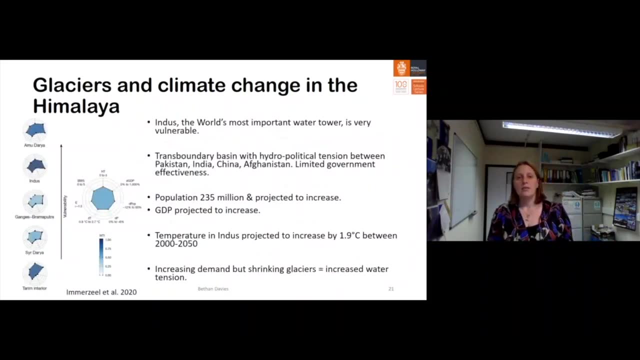 There is an unsustainable use of groundwater, So they are pumping up groundwater to fill the water gap. If the glaciers shrink and recede, the supply of water will decrease even further And these people will experience more severe water shortages. The Indus, which is the world's most important water tower, 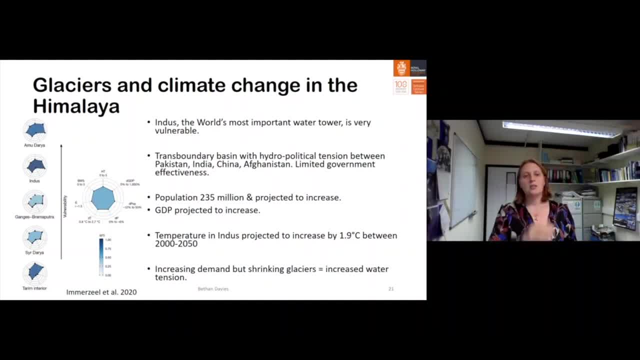 is also the world's most vulnerable. Here we have our spider diagrams again. In the Indus, which has a population of 235 million people, which is projected to increase, and is projected to have increases in GDP, we anticipate a large increase in the demand for this water. 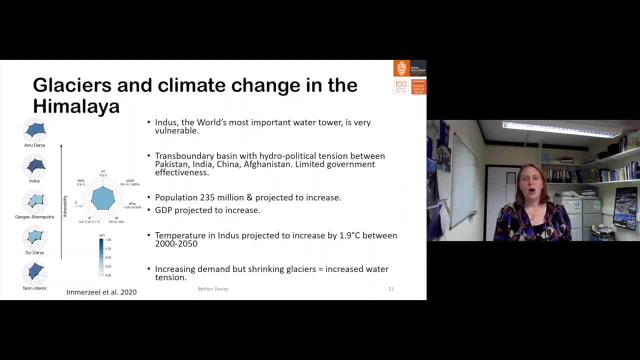 There is also a transboundary basin with hydro-political tension between Pakistan, India, China and Afghanistan. Governments need to work effectively together in a very volatile region in order to ensure that the water gap is not exacerbated in areas. downstream Temperatures in the mountain regions. 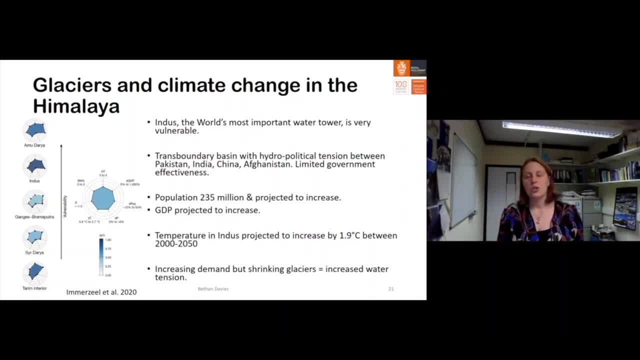 are projected to increase more than the global average, And that will contribute to increased melt in the Himalaya and will threaten these glacier water supplies. Ultimately, in the Himalaya we will see increased demand for the water but shrinking glaciers, which will lead to increased water tension in these countries. 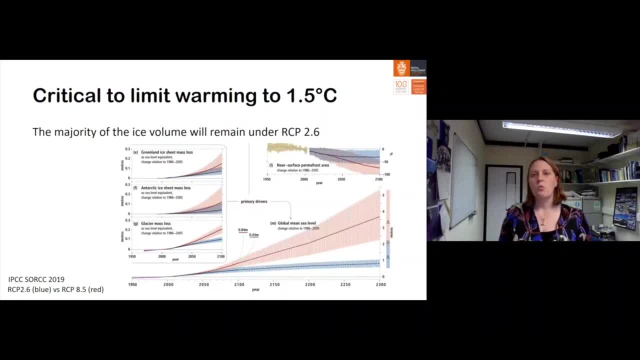 It is therefore critical to limit global warming to one and a half degrees centigrade. Here are a number of graphs. OK, so we've got Greenland ice sheet loss, Antarctic ice sheet loss and glacier mass loss, And then we have the global mean sea level. 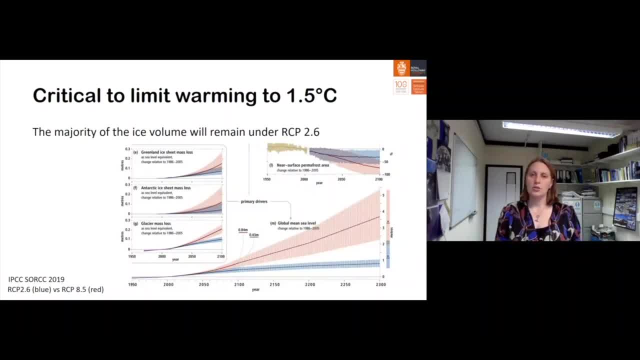 That's taken into account glacier and ice sheet mass loss as well as thermal expansion of the ocean. In red is RCP 8.5.. So in red we have the high-end scenario And in blue we have RCP 2.6.. 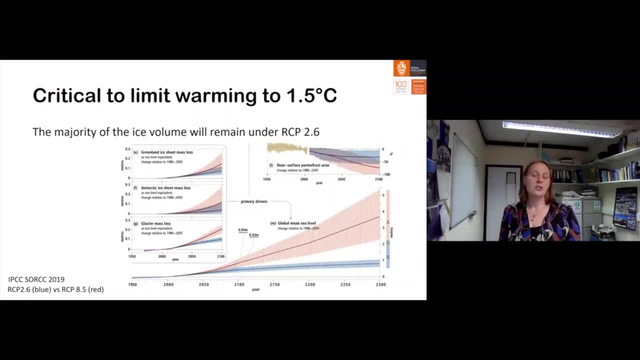 So blue is the low-end scenario: the Paris Agreement limiting warming to one and a half degrees centigrade. If we can follow the Paris Agreement by the year 2100, then we can see about 43 centimetres of sea level rise. 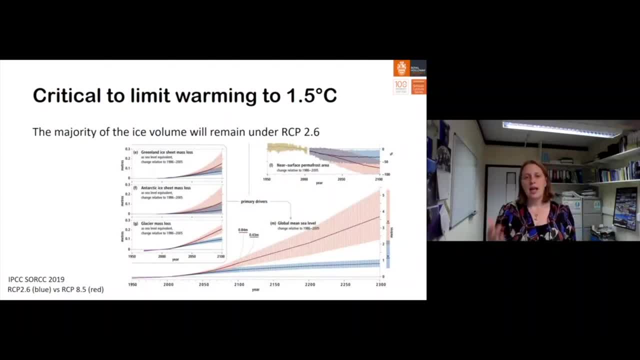 from all these different sources. Whereas under RCP 8.5, we can see a global sea level rise of around 84 centimetres under all these processes, By the year 2300, under RCP 8.5, global sea level rise could be around four metres. 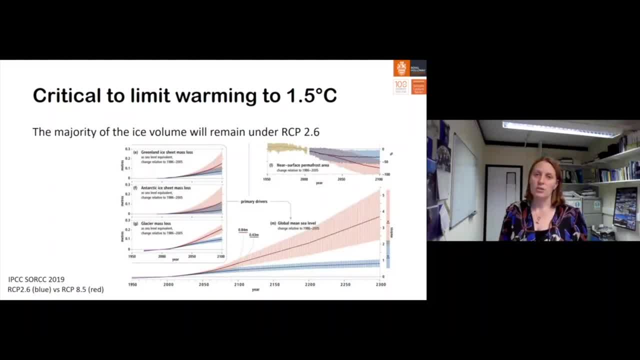 and almost all of the glaciers worldwide could be gone. We'll see perhaps a loss of the Western Antarctic Ice Sheet, significant reductions in Greenland and almost all glaciers will be lost. This is an unimaginable consequence that we must do everything we can to avoid. 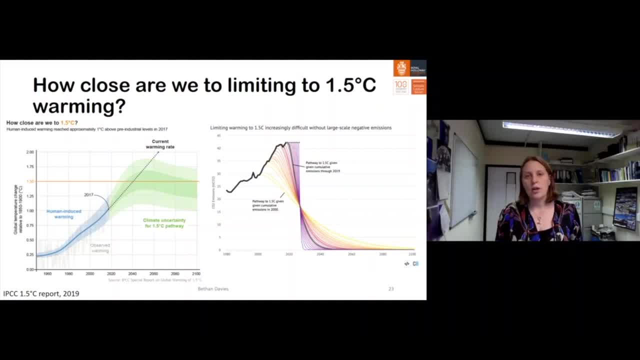 The pathways to limit warming to one and a half degrees centigrade become more challenging the longer we wait. You can see that the drop in CO2 emissions becomes increasingly steep the longer we leave it. The path to one and a half degrees centigrade is running out.